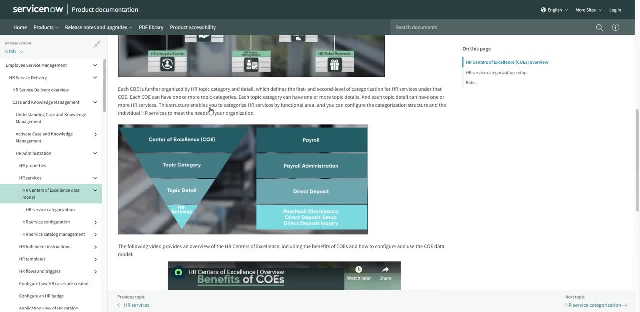 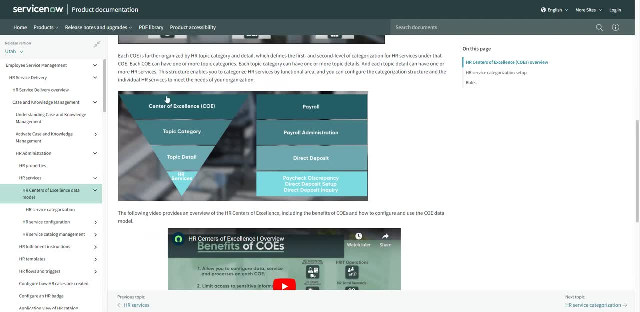 extended from the case table And this is just a way of organizing services into those Centers of Excellence. So this is a great diagram. here At the top you have the Center of Excellence. So in this example it's payroll, And then a Center of Excellence can have many topic categories. 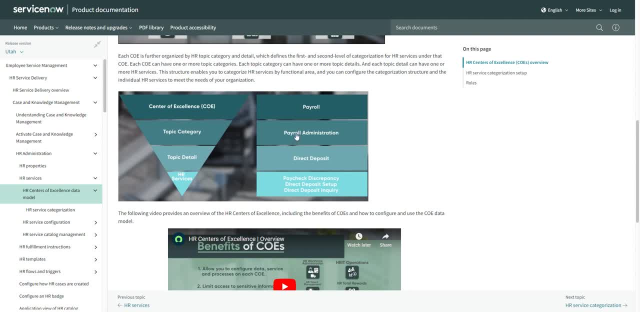 And one of those can be payroll administration, And then the category can have many topic details, which, in this case, is direct deposit, And then you'll have an HR service that's associated with the topic detail, which is associated with the category, which is associated with the Center. 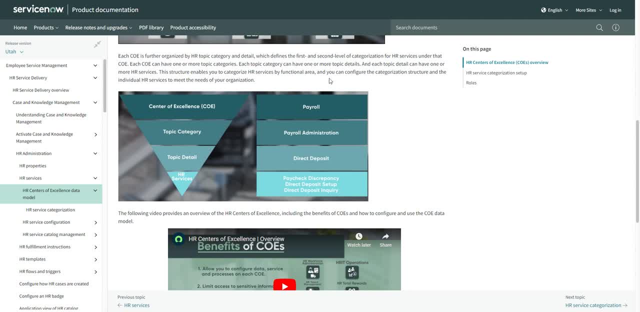 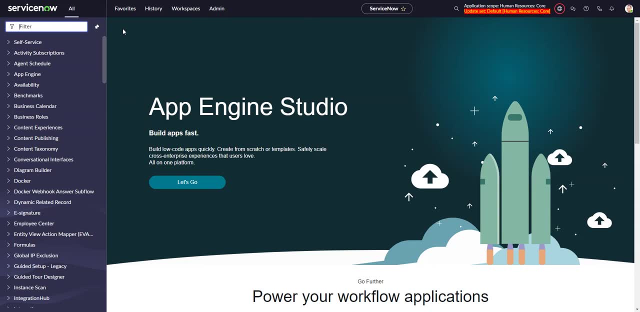 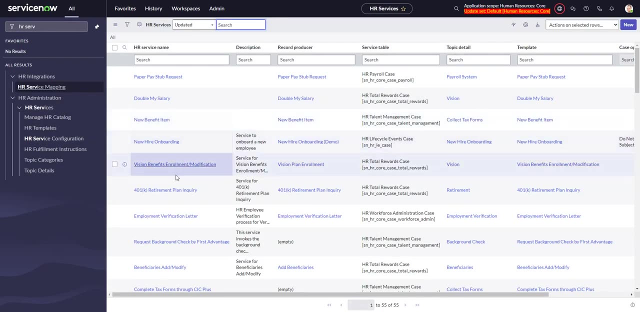 of Excellence. So that is structurally how it works. Let's take a look in the back end to see how this looks in the platform UI. So if we go to an HR service, let's take a look at the retirement plan inquiry. We can. 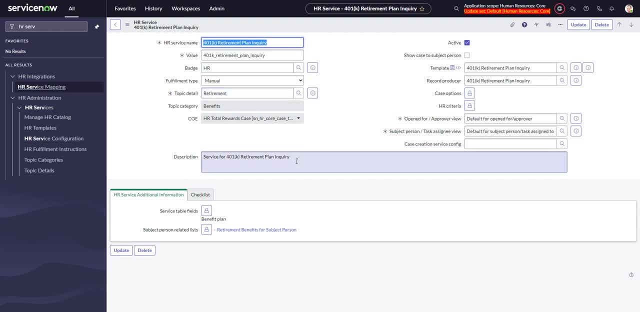 see that it is associated with a topic detail and then a topic category and a COE as well, And these fill in afterwards. So if we're actually if we're creating a topic, we're going to have a topic detail and then a topic category, We can see that you're creating a new one, sort of manually through. 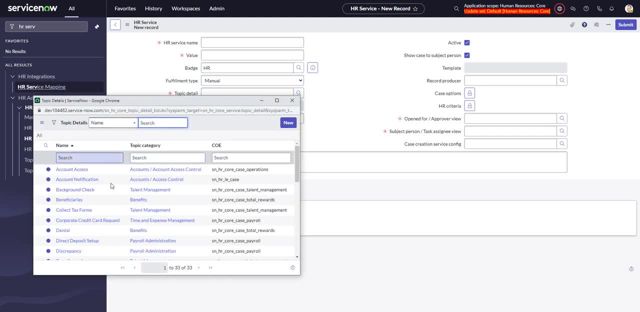 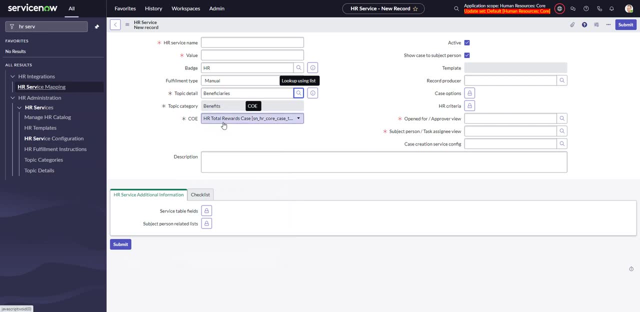 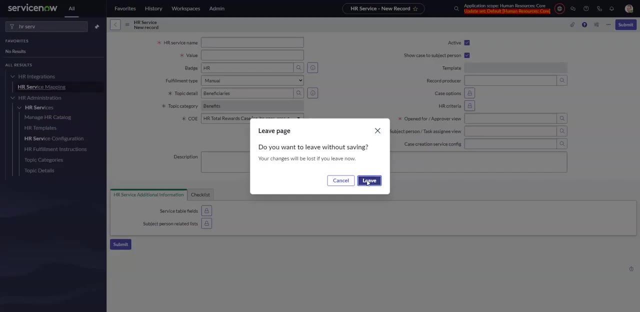 this UI and we go topic detail. We pick our topic detail, Say beneficiaries, And then our topic category and our Center of Excellence fill in automatically. The categories and the details can be managed in these modules. So there's a module for topic categories And this shows the category. 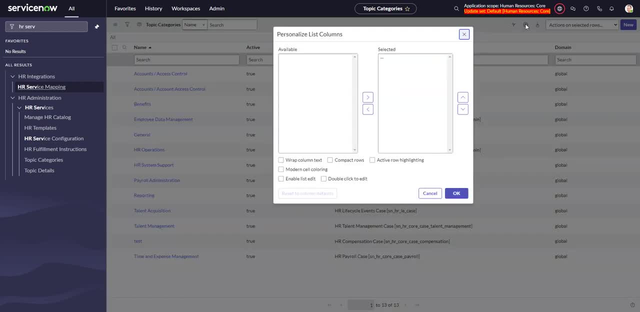 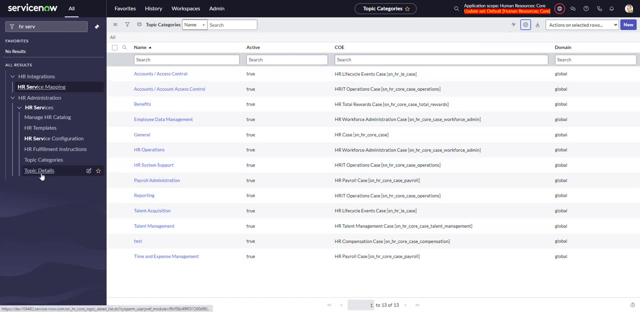 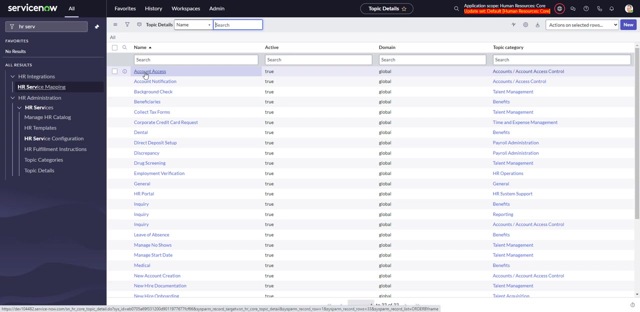 along with the COE, belongs to- and I think I'm in the default list view. yeah, I am, and this shows the the Coe that it belongs to- and then we have the topic details, and this is one step up in the hierarchy where we have the topic detail and then the 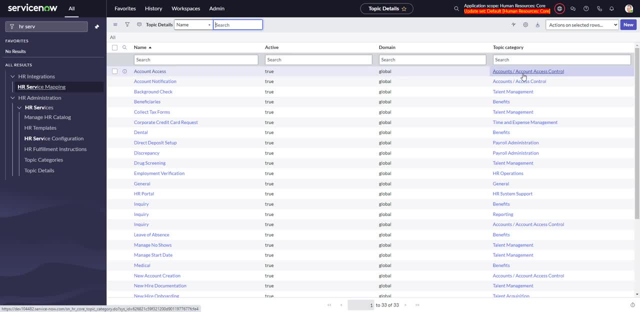 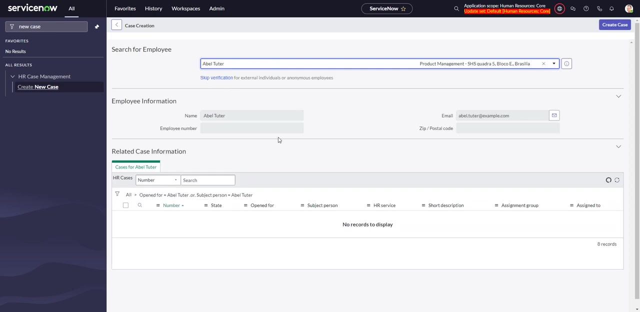 category that it's associated with. so these really are only destined for the for the fulfiller. the requester never sees anything with these topic categories and topic details and, specifically, if we're creating a new case as a fulfiller, let's pick on able tutor. it gets a lot of cases and I need 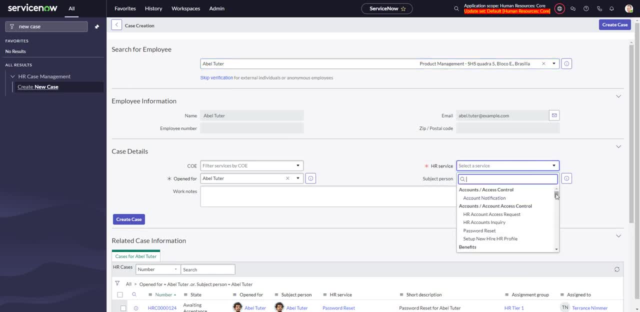 to select the HR service. the drop-down here has the categories as well as all the services under that category, so it's just sort of a way of organizing them. in my opinion, it's not super useful, because if I'm a fulfiller and I'm creating a, an HR case here, I'm probably 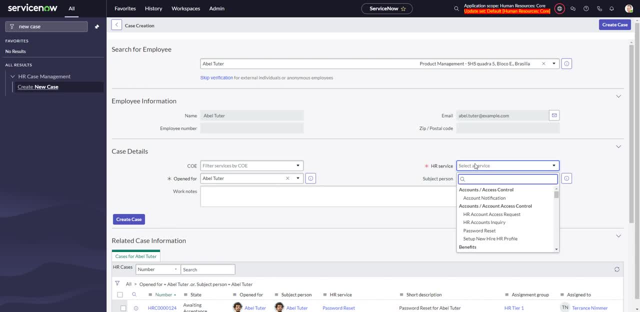 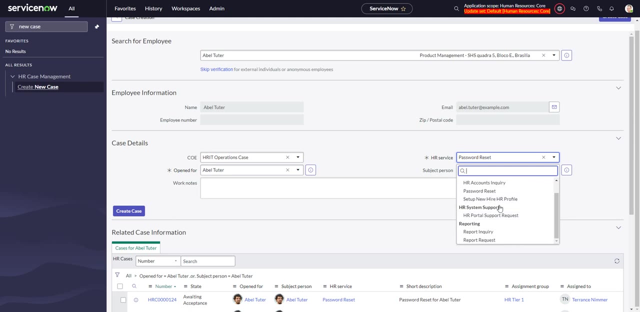 just going to pick the Coe, or I'm just going to type in my service directly, password reset say, and then my Coe fills in. so I don't. organizing it under the with the categories is not super useful, though I suppose it is somewhat useful you. 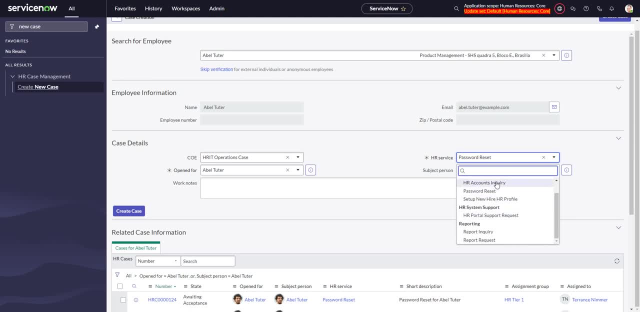 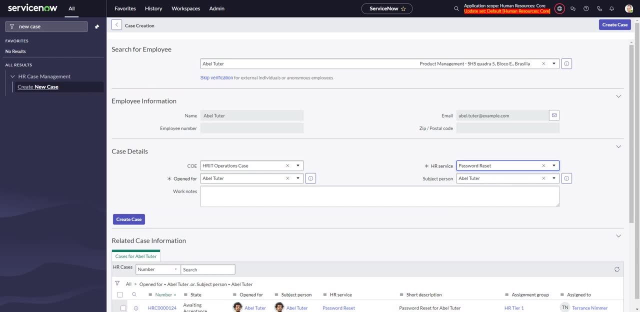 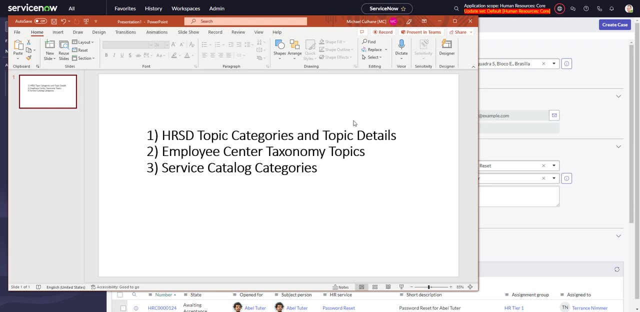 because if there are multiple services with similar names and you're doing a search, you can kind of see you what they belong to by looking at their category. okay, so that is hrst topic categories and topic details. the next organizational structure we'll look at is the employee center. taxonomy topics. 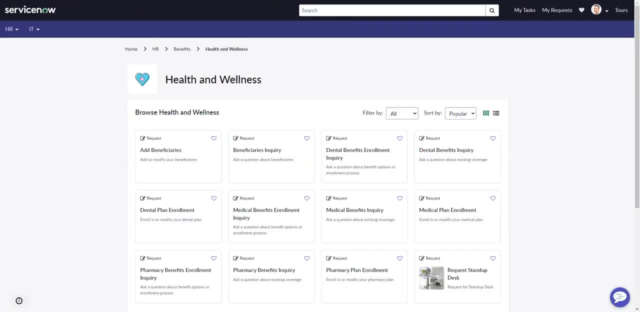 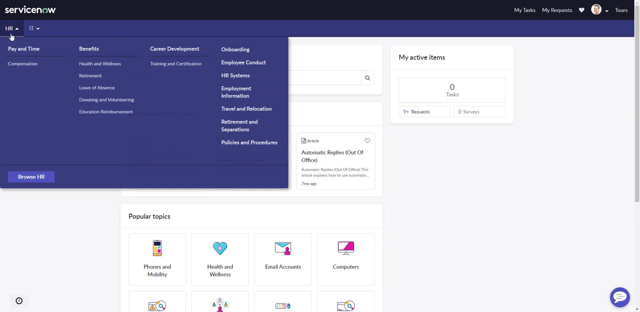 so this has to do with the front end, with the Employee Center and the different menu items that we see. an employee center. so in hr, out of the box, we have pay and time benefits, career development etc. and then another level down we have compensation, health and wellness etc. and so these topics are organized. 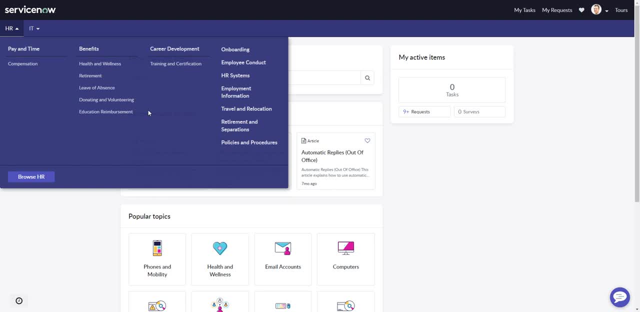 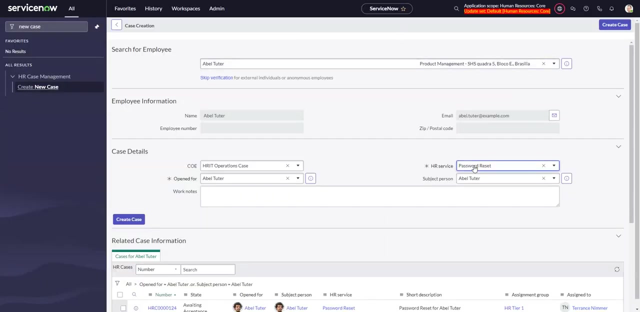 are also organized in a hierarchical fashion, but it is only topics. there are no topic categories and topic details. this one is just topics, and so what we're seeing here, although some of them have similar names, have nothing to do with what we see in here, or specifically, or specifically if we go to 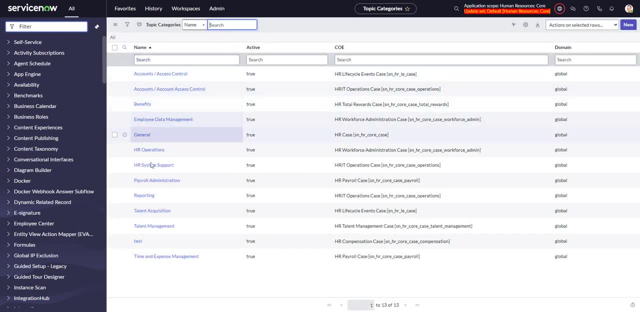 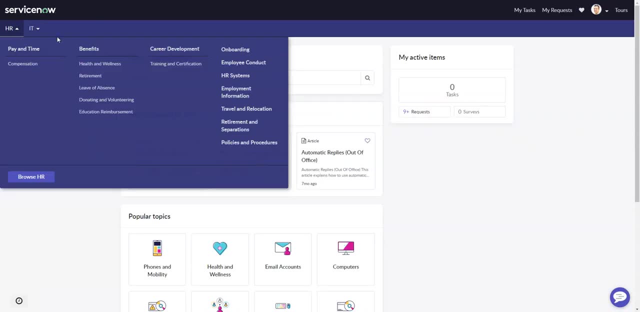 yeah, topic categories have nothing to do with this. even though there is a topic category called benefits and there is a a taxonomy topic called benefits, those two are independent and have nothing to do with each other. so these are in the back end. we can organize this with. 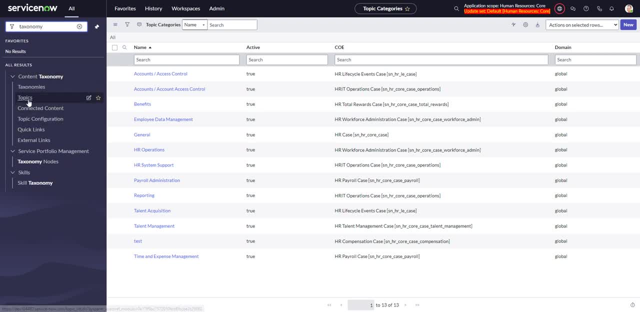 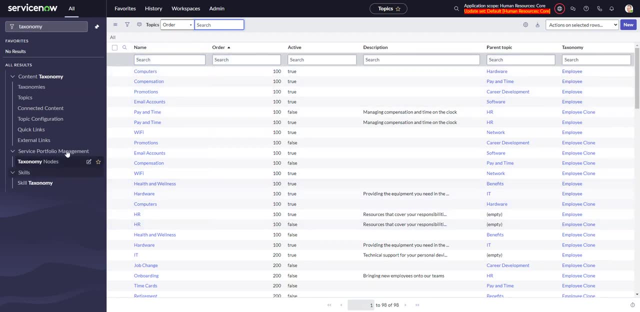 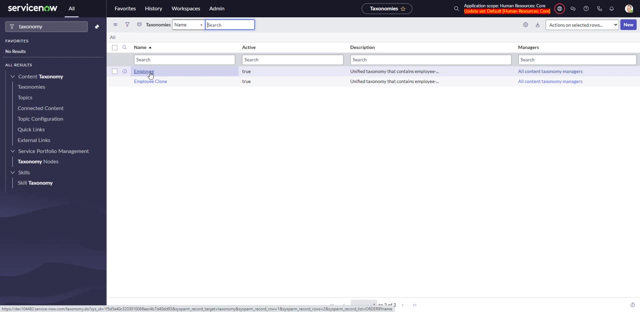 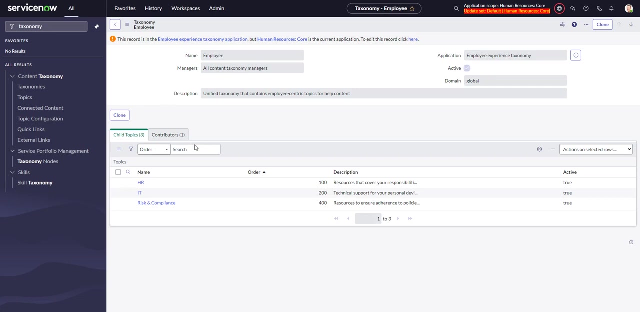 we search for taxonomy, we can see the topics, which gives us the hierarchical or the list of all of the topics. i find it more intuitive to go this way and go to your whatever taxonomy is being used by your um, by your uh employee center, and then i usually just drill down from there. so child topics: we can see hr and it. 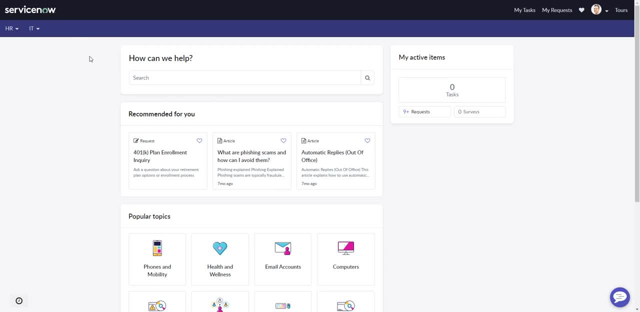 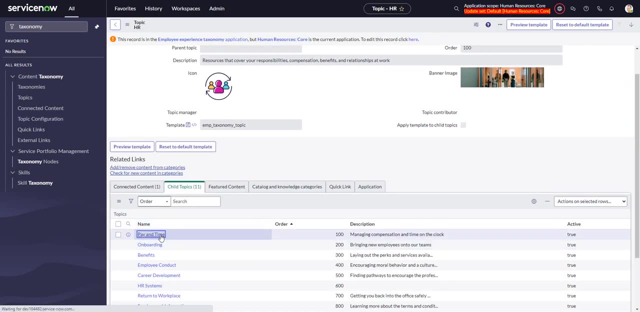 there's also risk and compliance. that's not showing up here because there are no items under there right now that are active. uh, so i drill down to hr and i drill down to pay and time, and then this is where i can put either content items or i can drill it even further down to more. 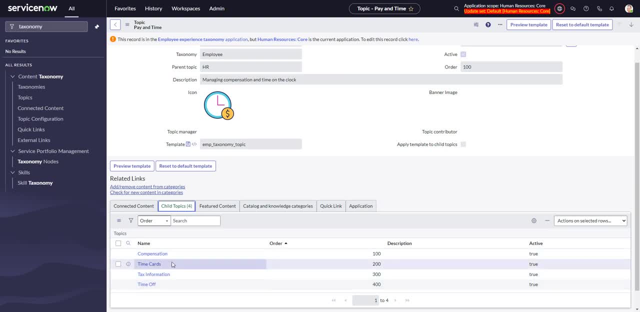 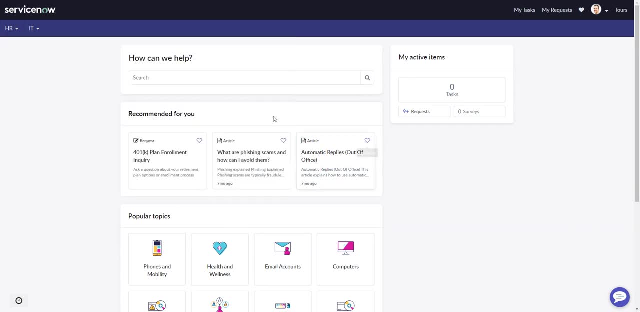 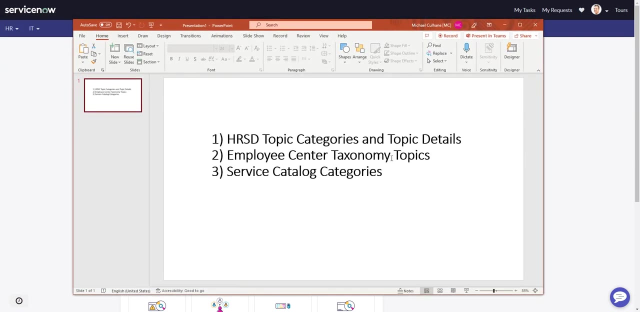 child topics and i have other videos that explain how to add content items under each of these categories or topics. i should say: keep my vocabulary straight. so that is employee center taxonomy topics which again, uh, can have similar names or the same names as top, as hrsd, topic categories and topic details. 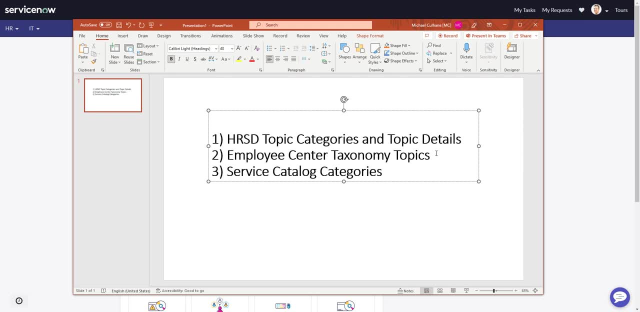 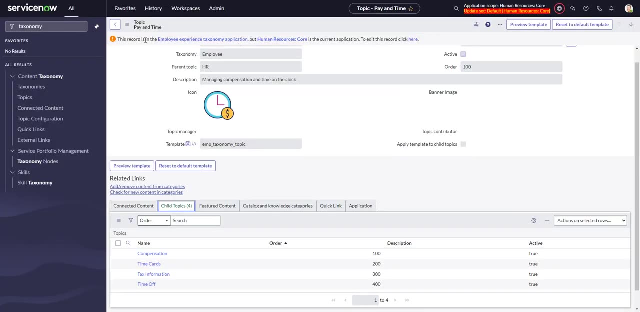 but technically have nothing to do with each other. there's no technical link between those two. and last but not least- uh well, yes, last and least actually is the service catalog categories. so these are from the service portal and, if you're familiar with itsm, they are much used in that application and 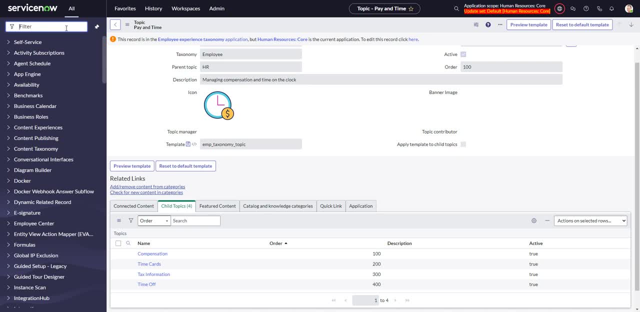 that product, but in hrsd in the current version, since employee center it's not really used anymore. so let's see where can we see this if we go to a record, actually let's do this inside of hrsd. so there is manage hr catalog, manage hr catalog. 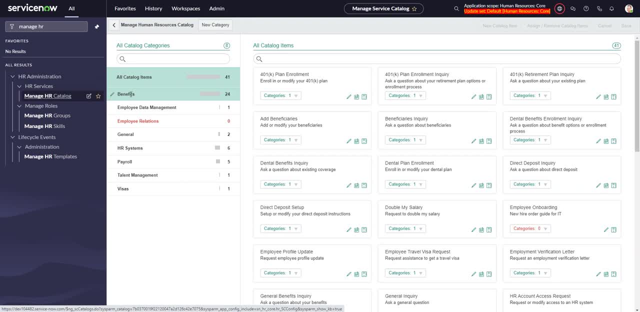 and there we can see the different catalog categories that are in the human resources catalog. so we have visas, talent management, payroll, etc. um, that's the place you would see it. but again you might think that, uh, hey, if i put it under, uh, if i put it under benefits here, well then,